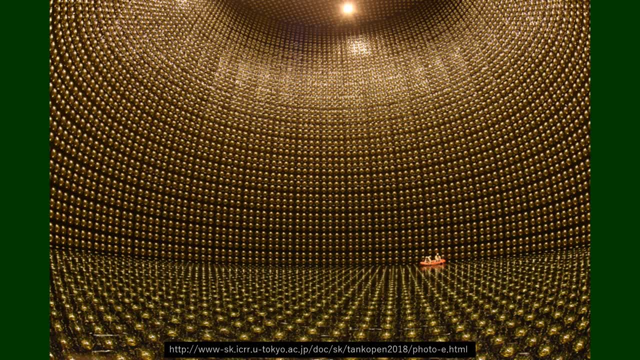 It also predicts proton and bound neutron decay, mediated by the new gauge bosons that connect quarks with leptons and quarks with anti-quarks. The original model was eventually excluded by searches at Super-Kamiokande and ELSP. We will describe the structure and some of the implications of the non-supersymmetric SU5 model. 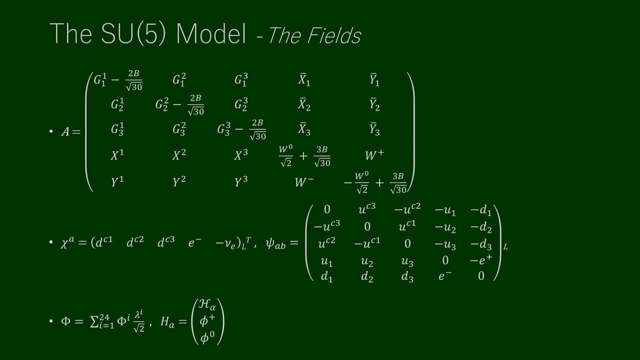 SU5 is a rank-4 group, like the standard model, with fundamental 5x5 matrices. The upper-left 3x3 block corresponds to the SU3 subgroup, while the lower-right 2x2 block corresponds to SU2.. There are 12 additional gauge bosons, X and Y, which carry. 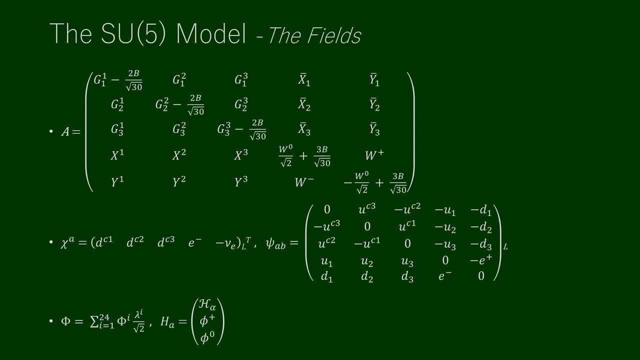 both SU2 and color indices. The 24 adjoint gauge fields can be written as a 5x5 matrix, where W and B are the SU2 cross, U1 bosons and G are the gluon fields. Each fermion family of left chiral fields is assigned to a reducible 5 plus 10 representation. 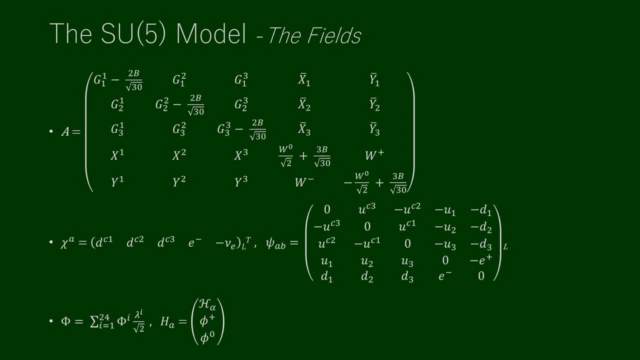 where the 5 chi is anti-fundamental and the 10 psi is the anti-symmetric product of two 5s, The field content can be written as a 5 plus 10 representation: where the 5 chi is anti-fundamental and the 10 psi is the anti-symmetric product of two 5s. 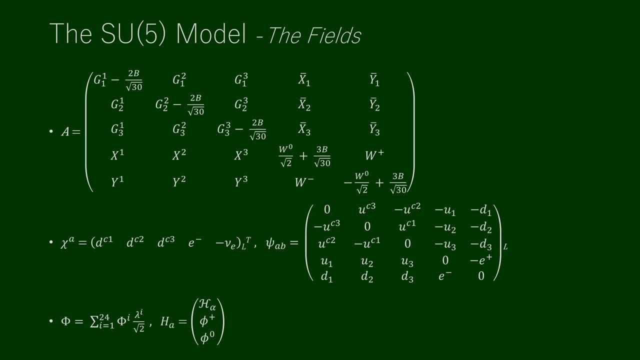 The field content can be written explicitly where the family indices and weak eigenstate superscript are suppressed. We also introduce a real adjoint, Higgs multiplet 5, and a fundamental complex 5-plet age that contains the standard model Higgs doublet. 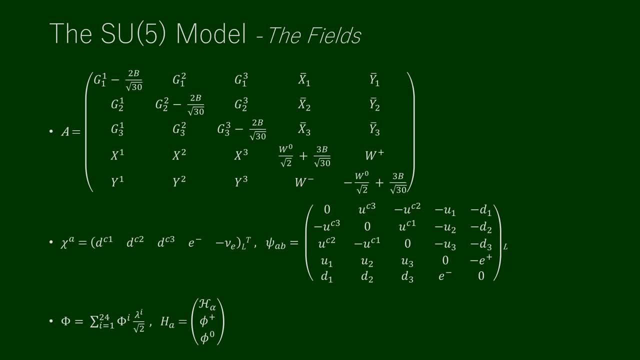 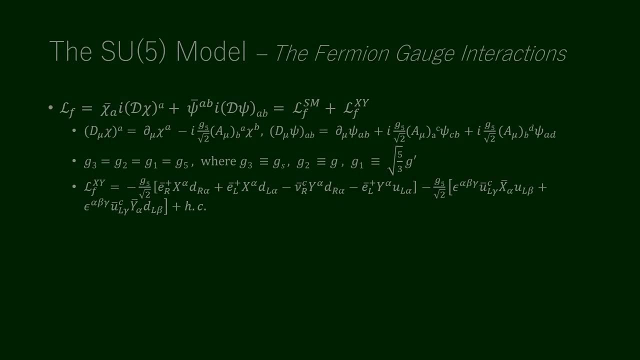 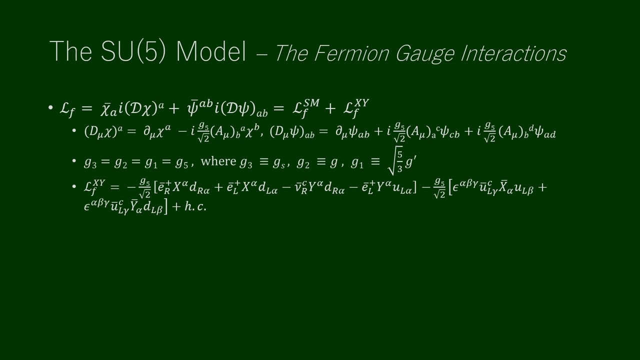 The 5 fields have the same quantum numbers as the gauge fields and are introduced to break SU5 down to SU3 cross, SU2, cross, U1.. The fermion gauge interactions are written where the fields are weak eigenstates and a sum over families is imposed. 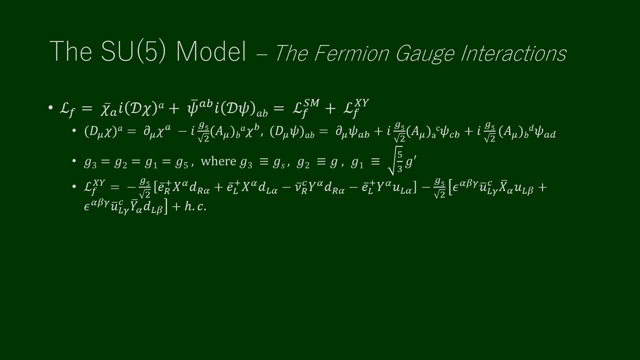 The gauge covariant derivatives are shown, where G5 is the SU5 gauge coupling. Lagrangian for standard model includes the kinetic energy terms in the standard model fermion gauge interactions with the restriction that the gauge couplings are unified. Lagrangian for XY contains the lepto-quark and di-quark interactions. 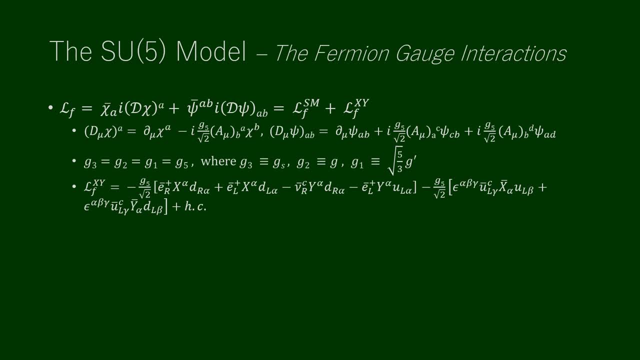 Lagrangian for XY contains the lepto-quark and di-quark interactions. Since the X and Y act, both as lepto-quarks and d-quarks, both baryon and leptron number are violated, leading to proton and bound neutron decay. 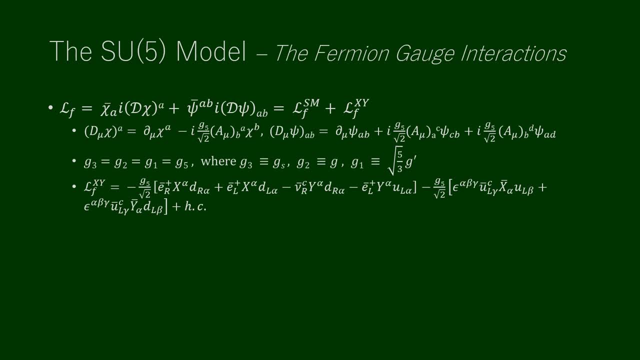 Prominent modes predicted by SU5 included: proton goes to positron neutral, pion, positron neutral rho, positron omega, positron eta and so on. The SU5 prediction of proton decay motivated a number of equations. Proton decay motivated a number of sensitive searches involving large underground detectors. 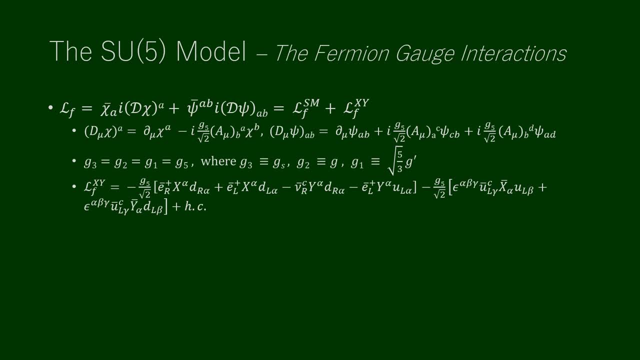 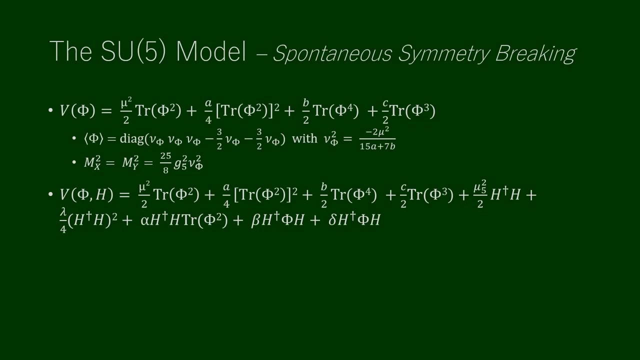 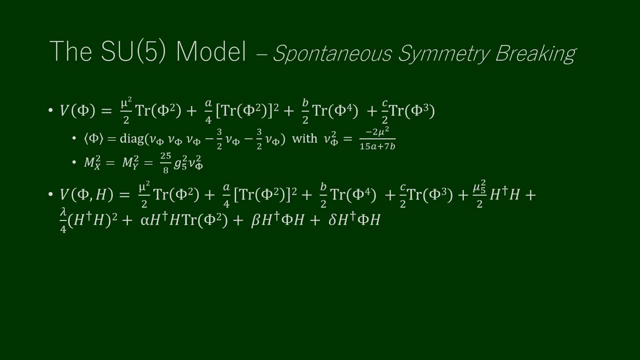 The adjoined Higgs. phi has a potential SU3, cross, SU2 cross, U1. at the guts cross, SU2 cross, U1 down to SU3 cross, U1Q. one must utilize the phi-plet HA. The potential for phi is extended where the SU5 indices are contracted in an obvious way and phi. 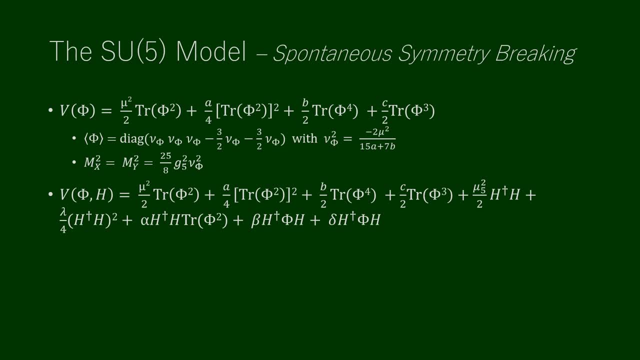 goes to minus, phi-invariance would imply: C equals delta equals zero. Two severe fine-tuning problems immediately arise: the gut hierarchy problem and the doublet-triplet splitting problem. Both of these enormous hierarchies must emerge from the parameters in phi-H.